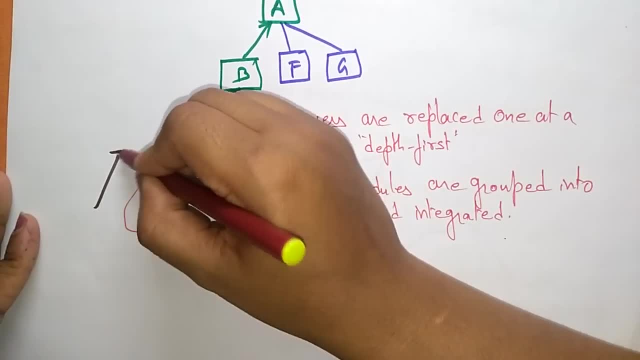 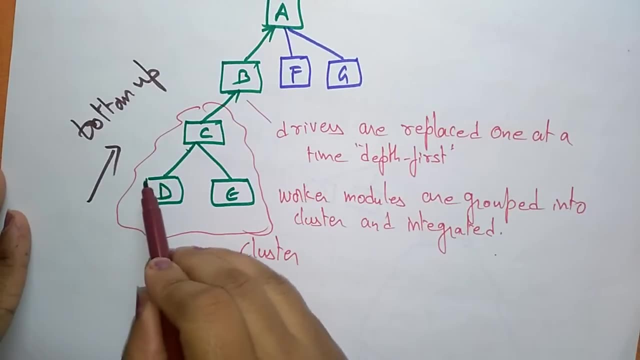 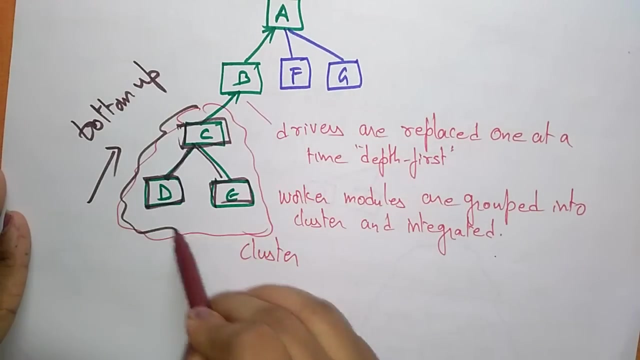 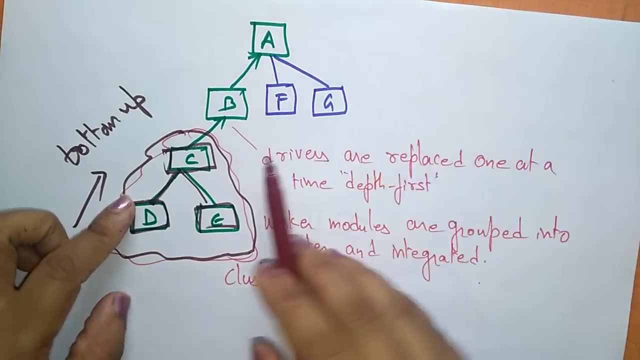 So here, first, it is following the bottom up approach. So in the bottom up approach, first you have to test the lower levels. The lower levels has to be tested and you have to be integrated and again you test on this higher level. So this complete system you call it as one cluster. Okay, This cluster will be replaced with this here in the drivers. So here drivers are replaced one at a time. 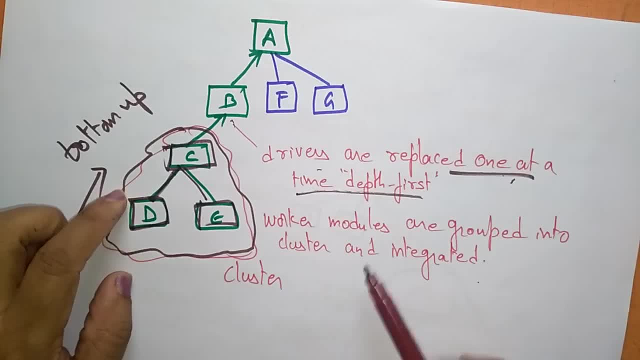 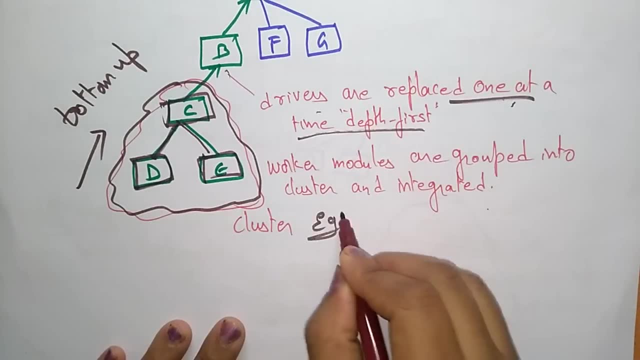 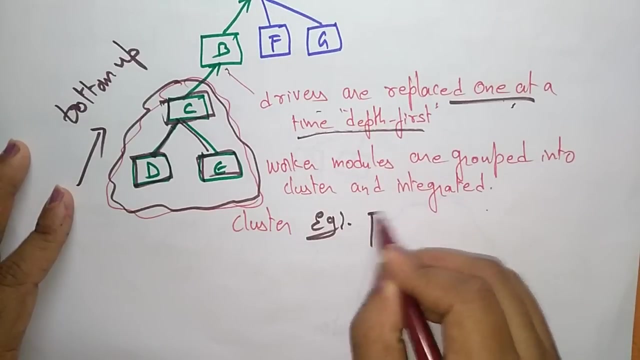 Okay, So the drivers are replaced, placed one at a time, the worker modules are grouped into clusters and integrated. so let me explain with another example. so, whatever the example i had taken in the bottom up, top down approach, so in the bottom up approach also, i'm taking: suppose this is a login page. 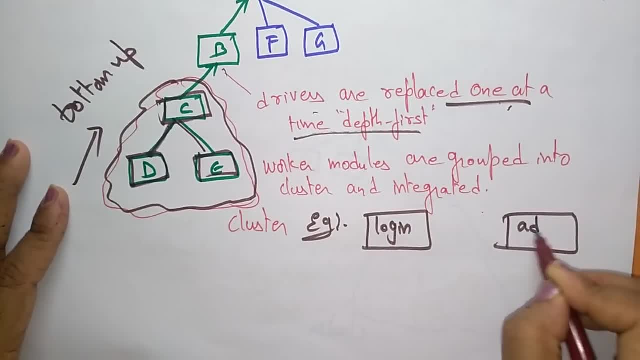 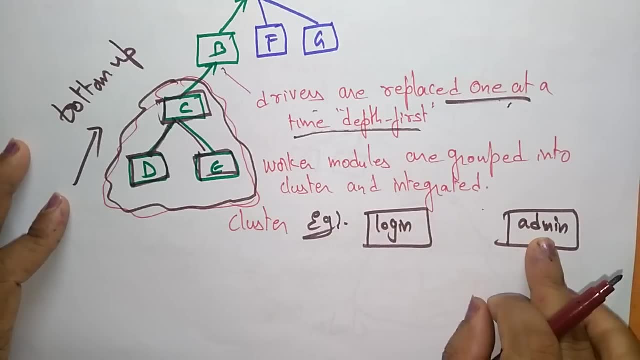 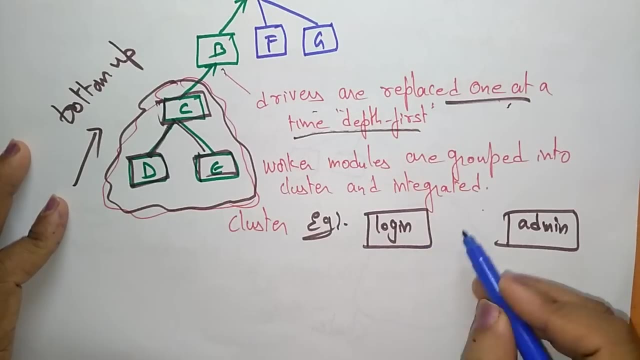 and this is the admin page. so there, i just called. the stop means the calling, that is a calling program admin page. now you here, we will take the reverse condition. let us take: the login page is not ready. okay, the admin is ready. the admin is ready for test, ready for testing. so admin page. 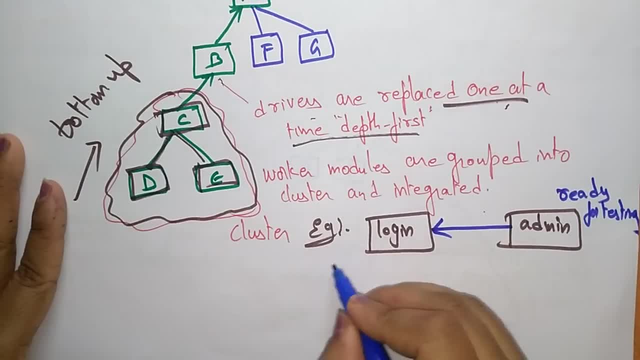 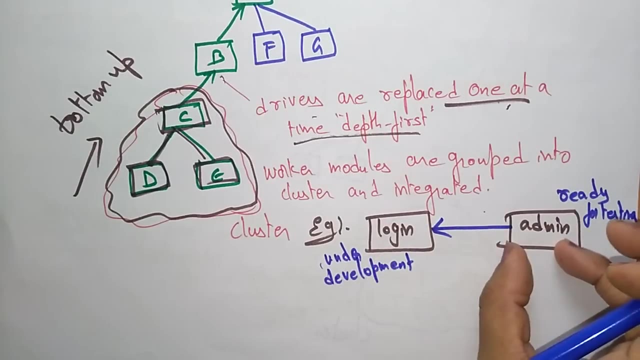 is over and it is ready for testing, but login is under construction, under under development, so whenever the admin wants to, you can see that the admin is ready for testing, so whenever the admin wants to, so whenever the admin wants to. uh called calling the login page means admin is calling the login page, but it is under development. 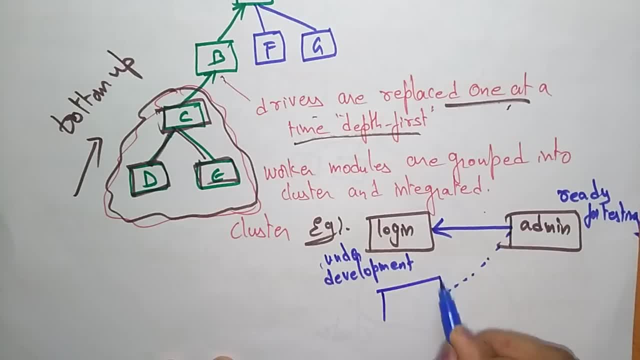 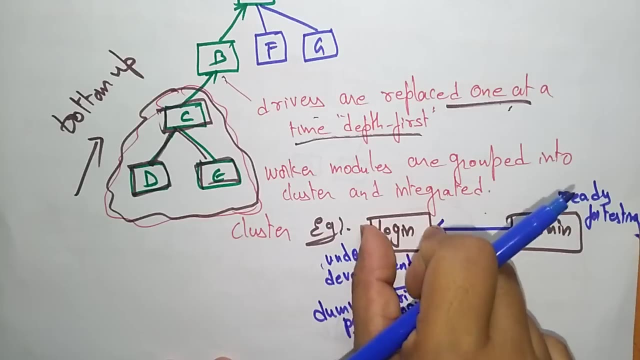 so it will be replaced with the dummy page. the dummy page you call it as a driver driver login page. so this is dummy page. so whenever the login is ready for testing, then this dummy page will be replaced with the exact login page. so that is a concept, that is the concept of the driver. 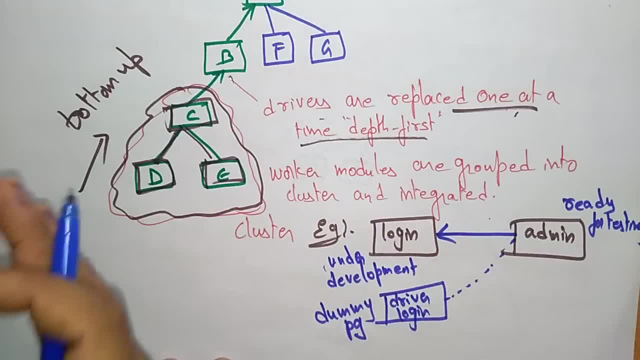 concept of the driver. so the driver will be used in the bottom up approach, and that uh, so the driver will be used in the bottom up approach. and that uh, so the driver will be used in the bottom up approach, and that uh stub will be used in top down approach. 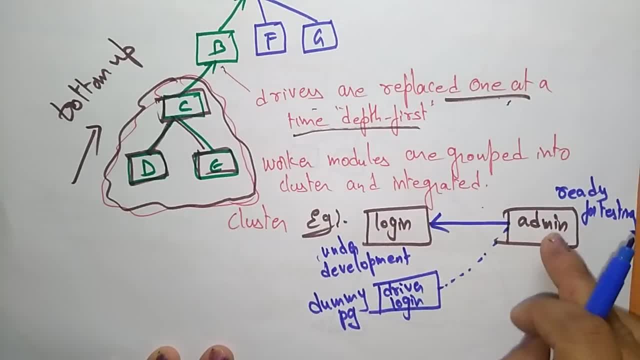 stub will be used in top down approach. stub will be used in top down approach. so here the calling if a calling program. so so here the calling if a calling program. so so here the calling if a calling program. so this is admin and here this is a calling. 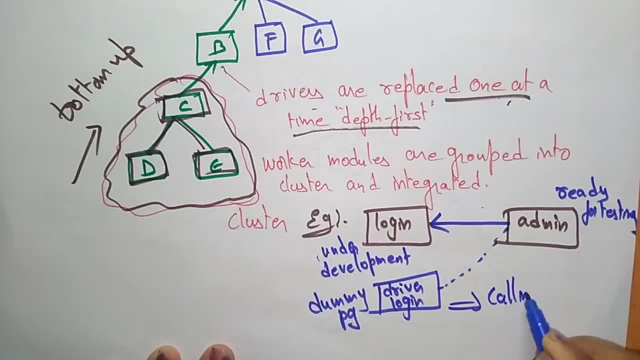 this is admin and here this is a calling. this is admin and here this is a calling program. the driver is a program, the driver is a program. the driver is a calling program. calling program. calling program. if the calling program is incomplete. so if the calling program is incomplete, so 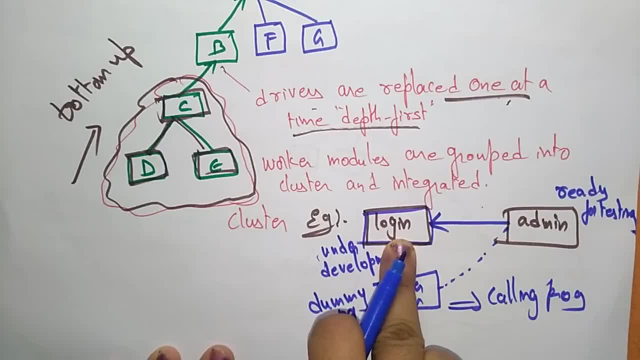 if the calling program is incomplete, so this is a login. if the calling program is, this is a login. if the calling program is, this is a login. if the calling program is incomplete, it is replayed. with a driver, incomplete, it is replayed. with a driver incomplete, it is replayed with a driver. this is it. 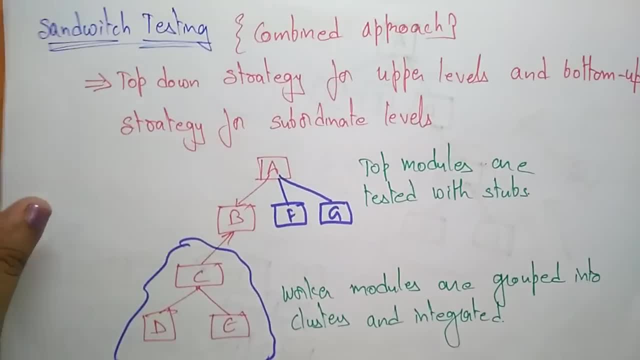 this is it. this is it. bottom up approach, bottom up approach, bottom up approach. and another sandwich testing will be, and another sandwich testing will be, and another sandwich testing will be there. that sandwich there, that sandwich there, that sandwich. sandwich testing is nothing, but it is. sandwich testing is nothing, but it is. 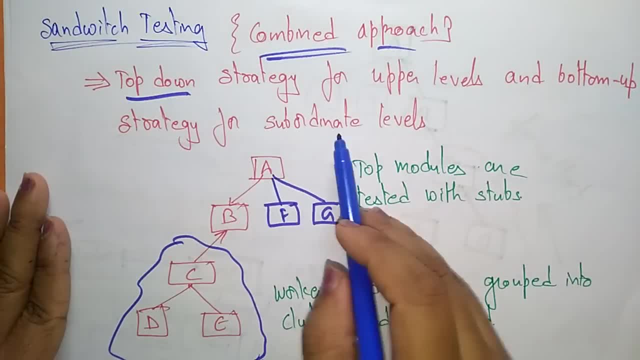 sandwich testing is nothing, but it is combining the true approaches. that is the combining the true approaches. that is the combining the true approaches. that is the top down and the top down, and the top down and the bottom up, bottom up, bottom up. the sandwich testing is combining the. 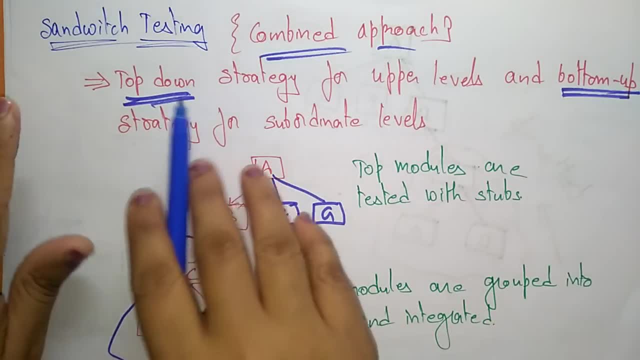 the sandwich testing is combining the. the sandwich testing is combining the approaches of both top down and bottom approaches, of both top down and bottom approaches, of both top down and bottom up. how it is doing the top down strategy up. how it is doing the top down strategy. 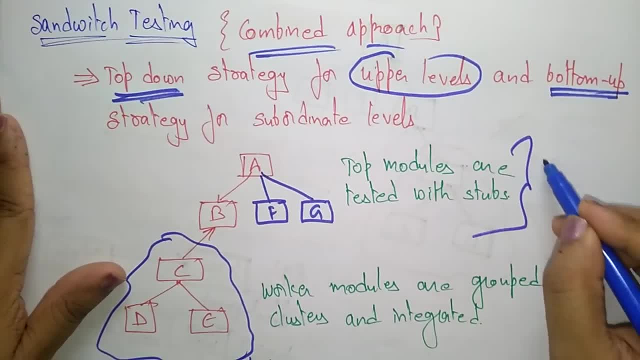 up how it is doing the top down strategy for only for upper levels, so upper levels, for only for upper levels, so upper levels, for only for upper levels, so upper levels. it is using the top down approach for upper levels, it use the top down for upper levels, it use the top down. 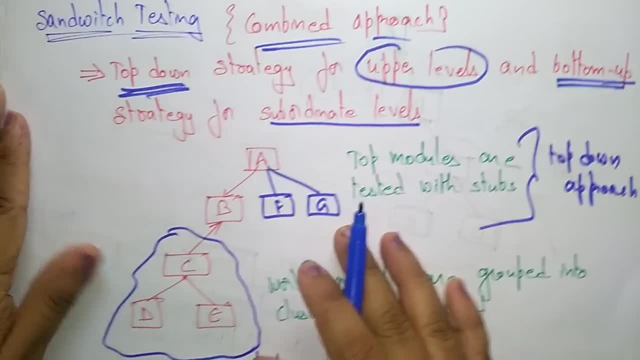 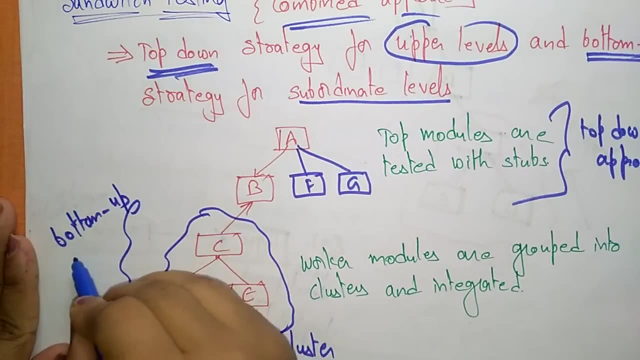 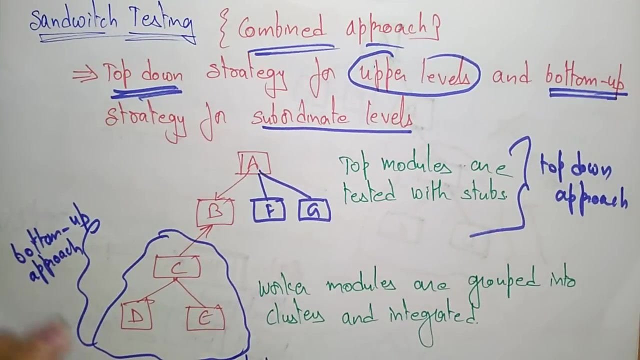 for upper levels, it use the top down approach and for bottom strategy, and this is bottom up approach. so the combination of two uh approaches, so the combination of two uh approaches, so the combination of two uh approaches is the sandwich testing, is the sandwich testing, is the sandwich testing. so these, the top modules, are tested with. 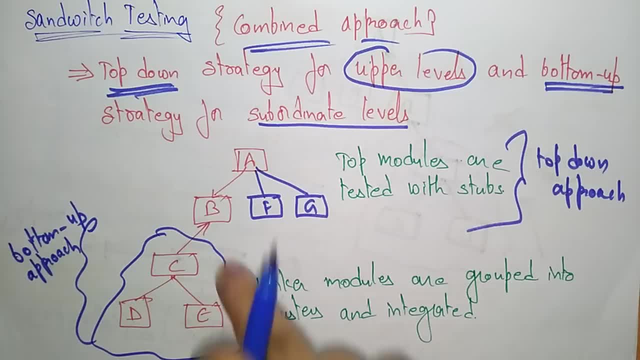 so these, the top modules, are tested with. so these, the top modules, are tested with stubs and the bottom will be tested with stubs. and the bottom will be tested with stubs and the bottom will be tested with the drivers, the drivers, the drivers. so it, after testing with the drivers, it 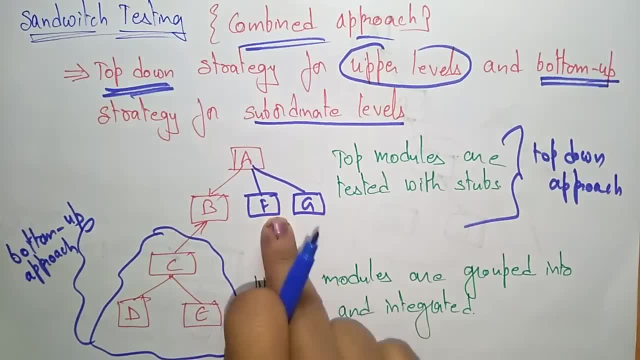 so it, after testing with the drivers, it so it, after testing with the drivers, it will be, will be, will be making as a cluster and this cluster will making as a cluster and this cluster will making as a cluster and this cluster will be replaced here and these top modules. 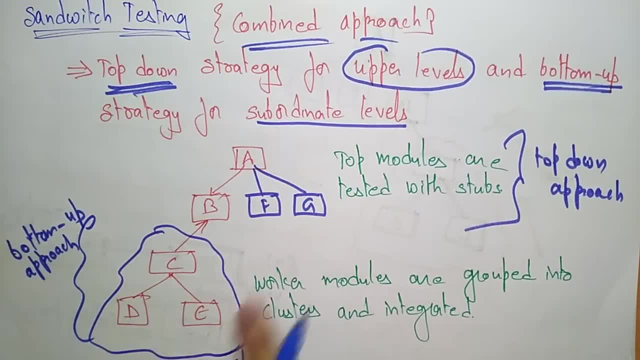 be replaced here and these top modules be replaced here, and these top modules are tested with the stubs until this will are tested with the stubs, until this will are tested with the stubs until this will be ready. after this uh is ready for: be ready after this. uh is ready for. 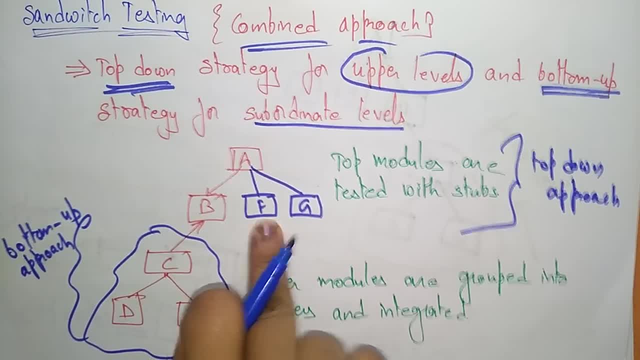 be ready after this. uh is ready for testing, then it will be integrated with testing. then it will be integrated with testing. then it will be integrated with this, this, this: uh, f and g. okay, uh, f and g. okay, uh, f and g- okay. so this is about the sandwich testing. so this is about the sandwich testing. so this is about the sandwich testing. thank you, thank you.